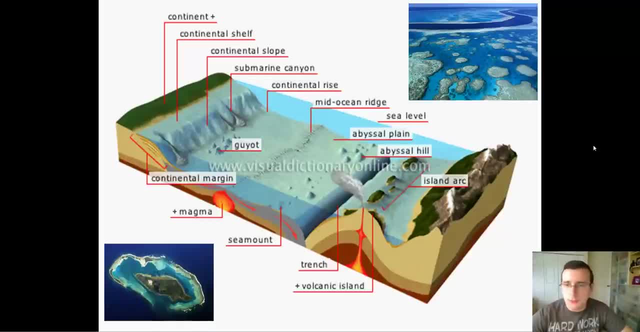 Alright, this video will focus on ocean geography, or topography or the shape of the ocean floor, But before we even get started on this, I want to talk about the difference between oceanic crust and continental crust. So some basic geology here. 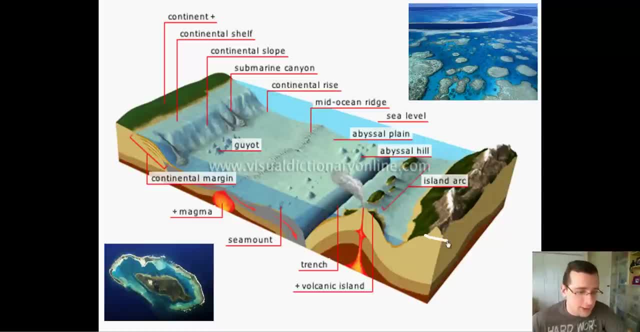 The continental crust is the crust that sits underneath a continent. As you can see, it is very, very thick. So you see, here the continental crust is extremely thick and it can be between like 5 and 80 kilometers thick. So it's very, very thick. 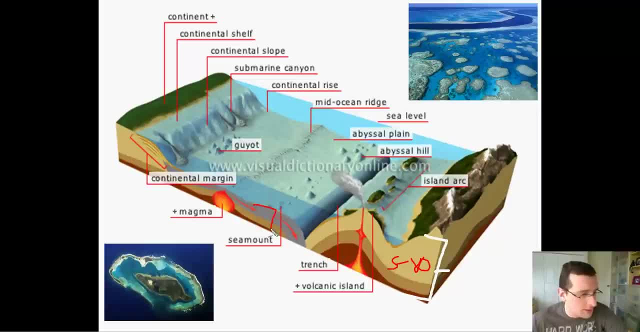 And now, meanwhile, the oceanic crust is very thin compared to continental crust, and it's only ever 10 kilometers thick, So it's much, much less thick than the continental crust is. So remember that the continental crust and the oceanic crust are different. 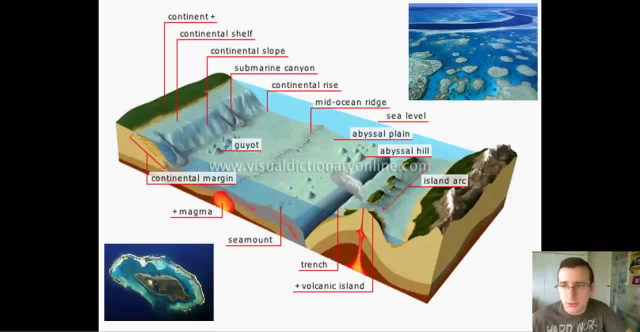 So what you see here? you see different plates in the screen And I'll show you where the plates split up. There's a split right here marked by the trench, Another split right here marked by the mid-ocean ridge, And then, which means that you have three plates or plate tectonics here happening. 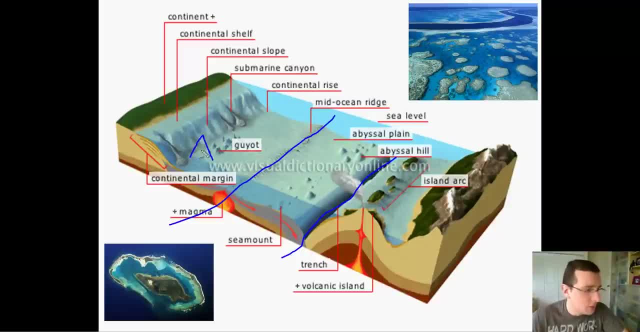 Three pieces of the earth's crust. Now, in this piece here, which I will call piece A from now on, the leftmost piece, you actually have both continental crust and oceanic crust on the piece. You see that there, On the piece in the middle- that's piece B- you only have oceanic crust. 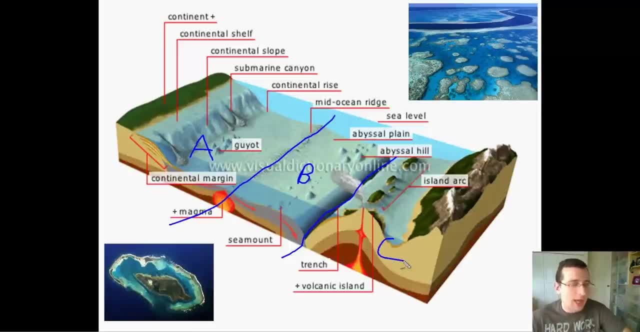 You don't have any continental crust. But on piece C all you have is continental crust. So you see how the crust of the earth, those tectonic plates, can be made of different parts. They can be made of both continental crust or oceanic crust. 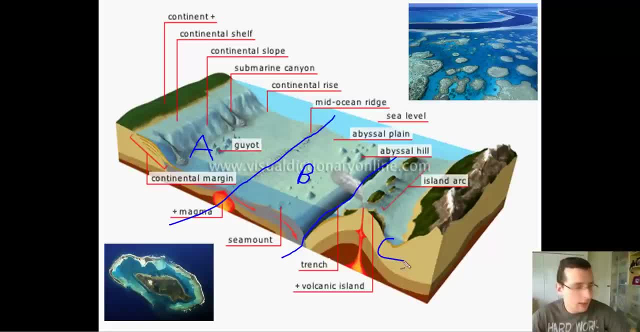 or just oceanic crust, or just continental crust. Now, when you talk about an ocean, how do you define an ocean? Well, we tend to define ocean by anything that's underwater, right? So the areas of the world which are vastly under salt water. 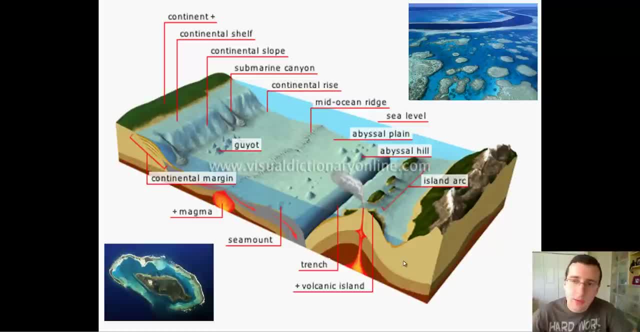 are usually considered part of the oceans, One continuous vast part of water. Now, if you think about it, that depends Why do you define it as a continent? Now, if you define it as a continent, the piece of land you can see- 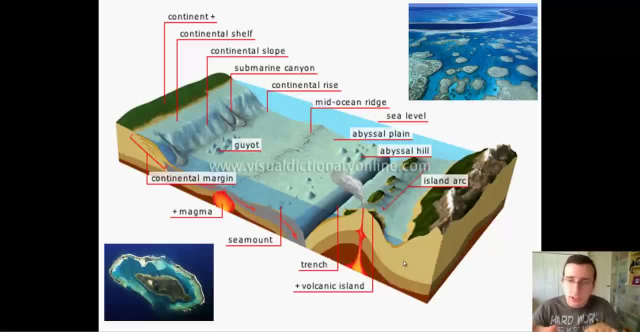 then you would have to say: the continent changes every day because the tides will be eroding the continent. the tides will be putting the continent on the water and then less on the water. That would mean the continents shrink and stretch over day. 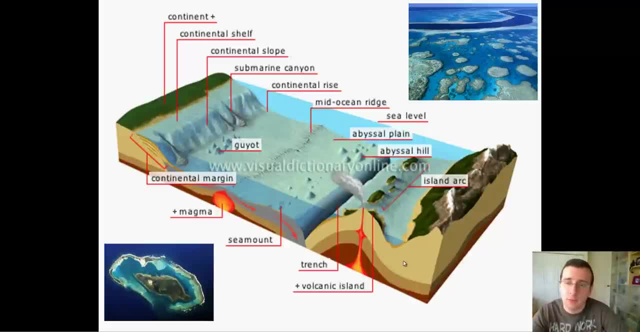 That doesn't make any sense. So the formal definition of a continent is a continental crust. So if you are part of a continent, that means that you are going to be one continuous, continuous continental crust. So this right here, all the way to the end of the continental crust. 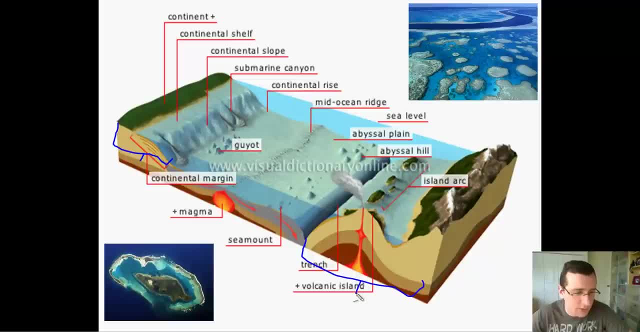 will be considered part of a continent and all of this will be considered part of the other continent, And that's the geological classification of the actual continental body. Anything that's part of the continental crust is automatically part of the continent. That means that some of the continent is actually part of the ocean. 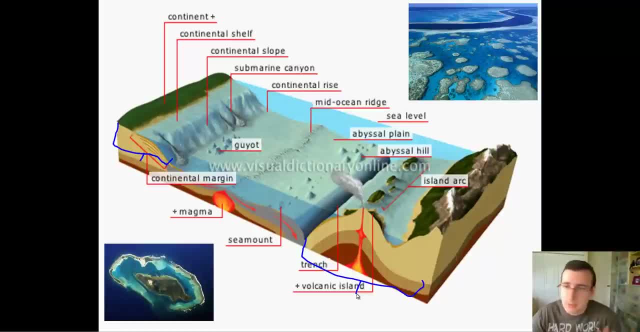 That means underwater, And that's something that I wanted to clarify. So there are two main parts of the ocean. There's the ocean parts that belong to oceanic crust, Or in other words, parts of the ocean which are deep underwater and are part of oceanic crust only. 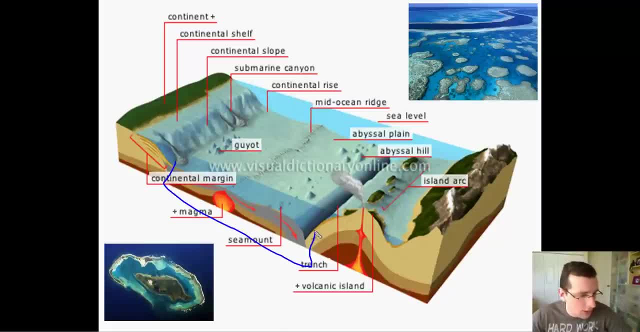 So, for example, from here all the way to here, that would be considered oceanic crust only And that we call a deep ocean basin. Now there's also ocean parts which are actually above continents or continental crust, like this piece over here. 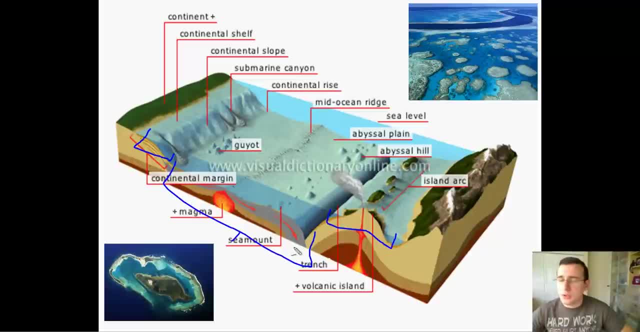 or this piece over here, And those we call continental margins, which are the pieces of the ocean which are above a continent. So when you think of a continent, you're going to think of the part which is above water and the part below water. 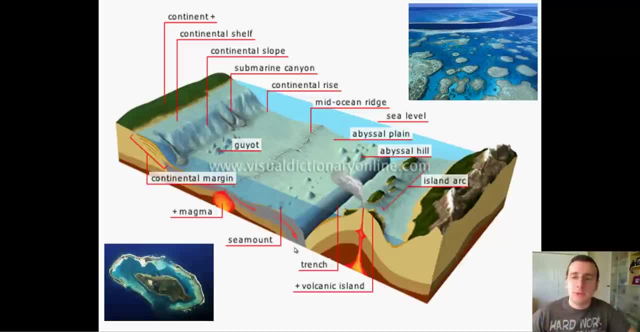 which is also part of the continental crust, In other words, the continental margin. Now let's talk about the structures of the ocean floor. The continental margin, which is the part of the continent underwater, actually splits into three different parts. You have the continental shelf. 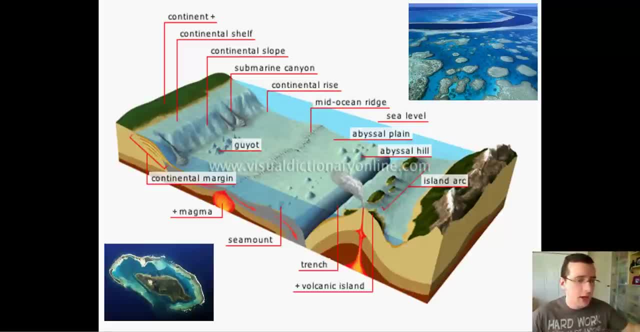 the continental slope and the continental rise, And you see there that on the top left-hand corner. Now I'm going to start on this side. This is also continental crust, but I'll talk about this side because it's a little simpler. 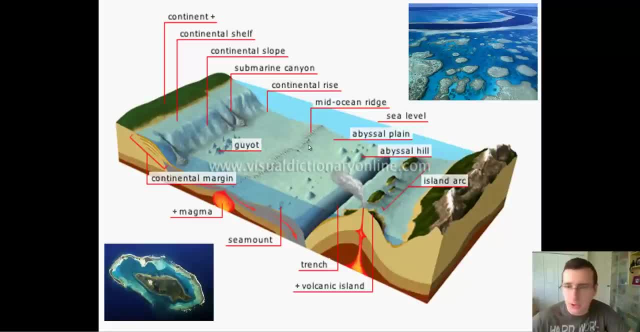 Now the first most prominent feature of the continental margin, which is part of the ocean, is called the continental shelf. To explain the continental shelf, I have to draw a square, So give me a second. So imagine for a second that this box here. 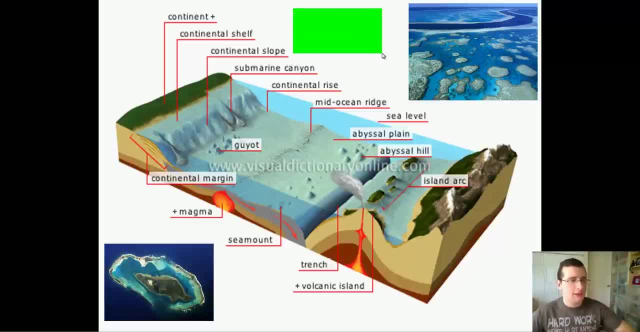 represents an ancient continental crust. that was there, not necessarily covered by ocean, And then you're going to have on the other side, the ocean is going to start coming through and actually waves are going to be hitting this constantly and it's going to start eroding this. 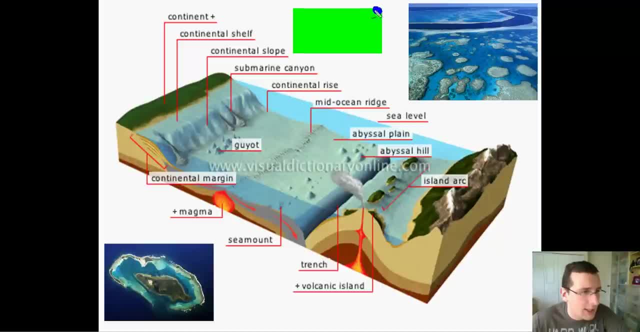 And so the waves are constantly hitting this, eroding it and cutting chunks out of it. Before you realize, you start getting this slope here. Now, obviously, the waves will go into a certain depth, So it can't erode more than that, right. 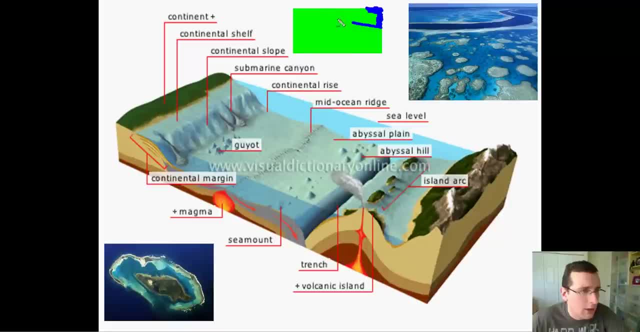 But with time, the waves will more and more destroy the continental piece, But it will never go lower than this, because the waves will never go lower than this. And so, while this process will continue in this direction and the continental erosion will continue over time, 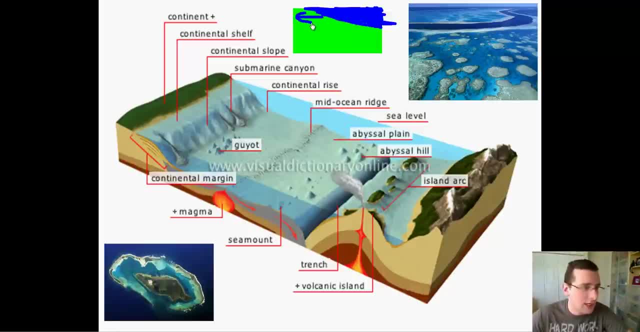 and then, over time, you're going to get more and more continents disappearing because of the motion of waves constantly hitting the continent And you're going to erode it. You're never going to get below this point, because that is as deep as the waves will go. 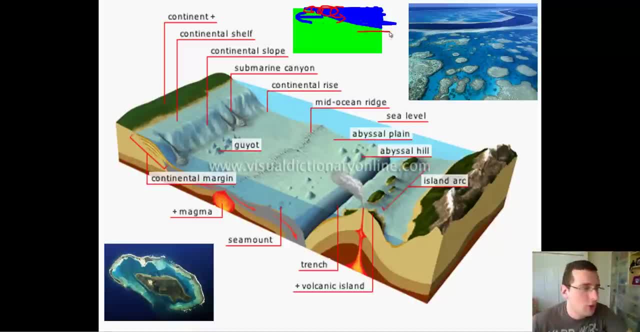 And so what you end up getting is that there is this steady slope below the water, which is called the continental shelf. Now, eventually, when you get to that point where the waves no longer act, you get a sudden drop-off where the shell just goes. 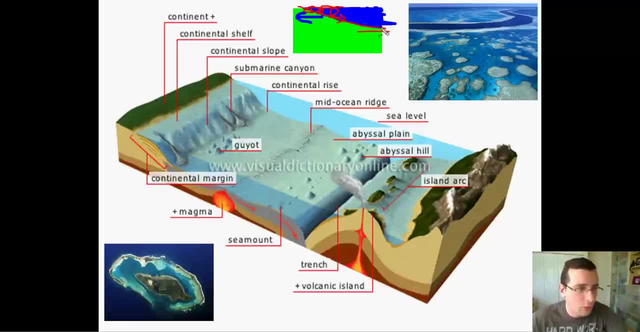 boom all the way down to the bottom of the ocean And that we call the continental slope. So the continental slope is right here and the continental shelf is this steady incline towards the continental slope. When you get to the slope it's a sudden dip. 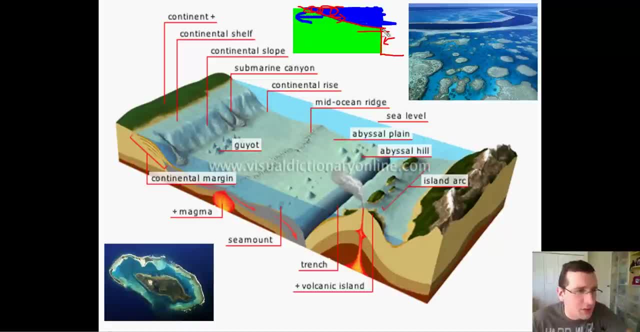 of the actual slide. So you might end up over time getting a bit of a slope that's much more steady than the continental shelf would be. And why is it you're getting this gradual slope Because of landslides Now, ever so often. you see here in the picture. 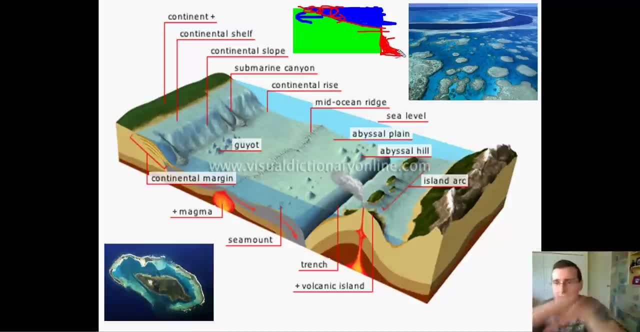 you're going to get a landslide, where the continental shelf will, because of an earthquake, will destabilize and will collapse and form a landslide. By the way, whenever that happens, all that dirt that's coming from the continent mixes with the water in an instant. 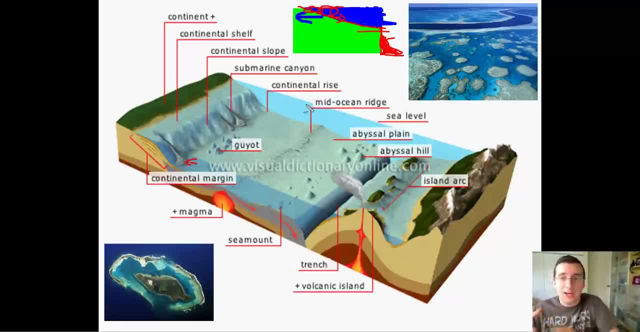 and it causes what is called a turbidity current. This is murky brown water that actually pushes all the water forward and actually causes a tsunami. So one of the things that causes tsunamis is the collapse of the continental shelf. Now, as the continental shelf collapses, 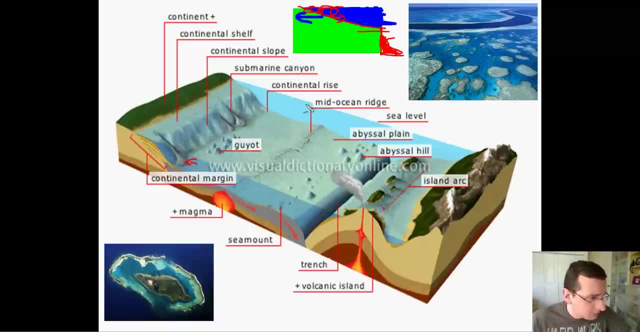 you actually get these gaps in the continental shelf, which are called submarine canyons, And these gaps went on to become a bunch of sediment that gets thrown into the deep ocean basin to create this slope that I'm talking about here. It's a bunch of sediment, that's really. 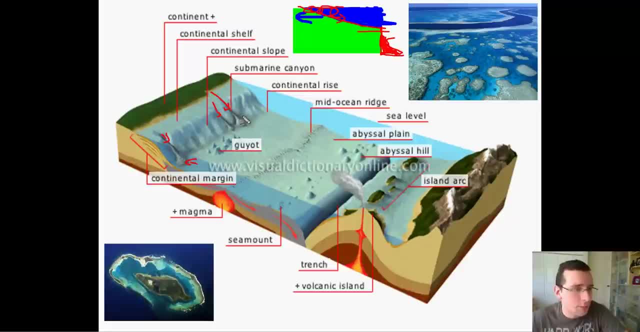 all coming from the collapse of the continent. That is what we call the continental rise. So, for review, the continental slope is the steady decrease of the continental shelf because of wave erosion. The continental slope is the sudden deep dip as the continental shelf ends. 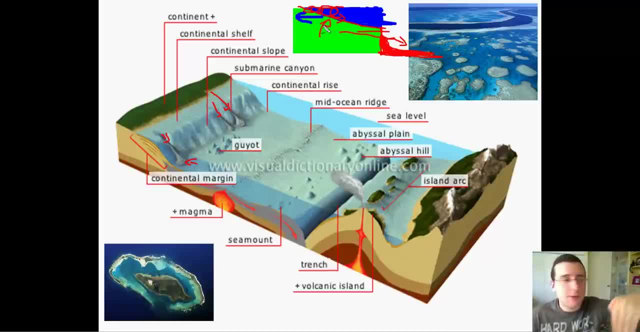 And it's sudden because that's the area where the continental shelf ended, but there's no erosion happening there. And then you have the continental rise, which is the accumulation of landslide material over centuries of destabilization. So you have a lot of destabilized continental shelf. 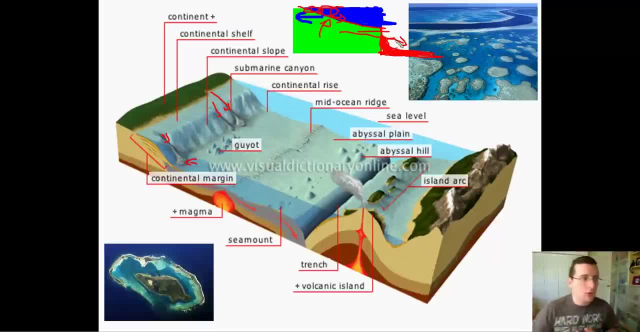 creating canyons and turbidity, currents and things like that, And that, in a nutshell, is your continental margin, which will include features like the continental shelf, the continental slope, the submarine canyon and the continental rise You also may have sometimes. 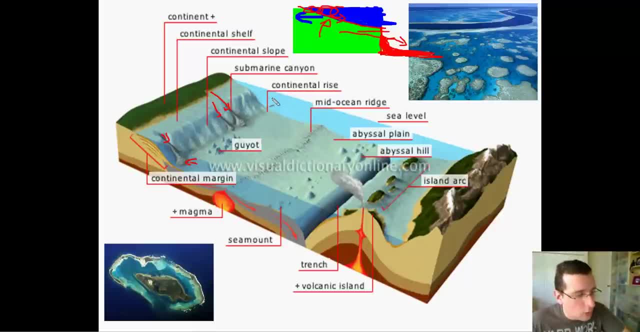 something called an island arc. Now, an island arc it forms on the opposite end. When an oceanic crust collides with a continental crust dead on like this, you will form a trench in between, But this causes the continental crust to actually bulge up like you see here. 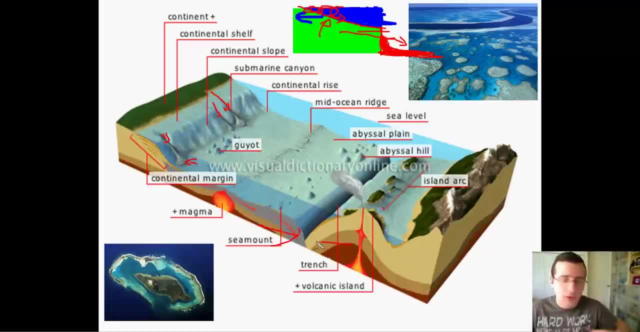 And this bulge will create cracks and things like that, which will create a series of volcanoes and mountains underwater which may actually protrude over the top and create an island arc or a series of islands away from the continent. So you actually see an island arc. 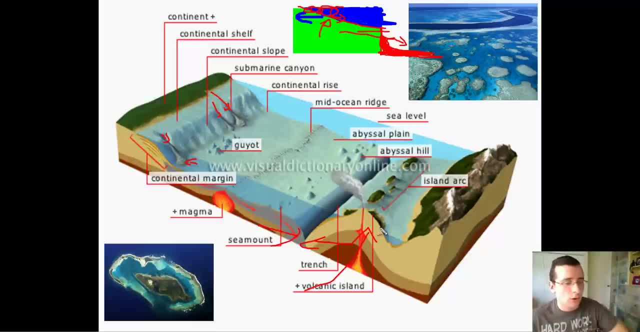 and then you actually see the continental rest. So this is an example. This on the right side with plate C is what would have plate A if it were to collide with an oceanic crust, And so that's not happening to plate A.